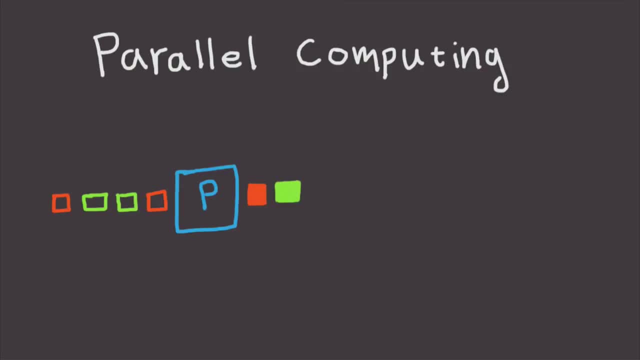 going to discuss in this video. But let's have a look at traditional computing, The type of computing which is not parallel. So we have the processor here and the instructions come in and the processor does the processing, and then you have the processed data here, As you can see, 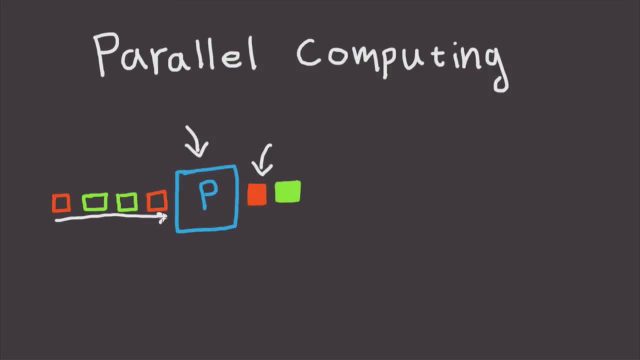 there's a queue of new instructions coming in and the processor is doing its job and then we get kind of processed data out of it. Now there's a problem with this approach, especially in the past couple of years, and the problem is that we can only 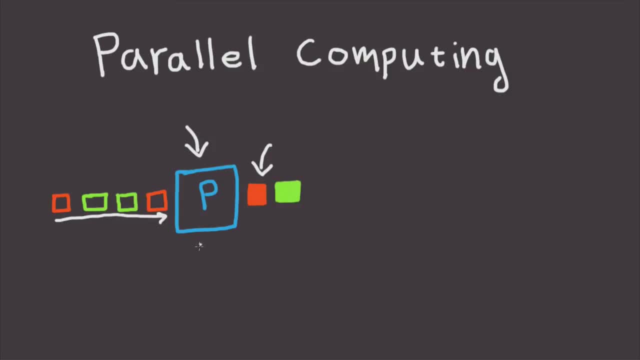 make this processor faster to a limit- There is a frequency limit- and the reason? there are plenty of reasons actually, but one of the important ones is heat, because these processors are very, very kind of condensed, so the amount of heat generated by electrons moving through the processor is very 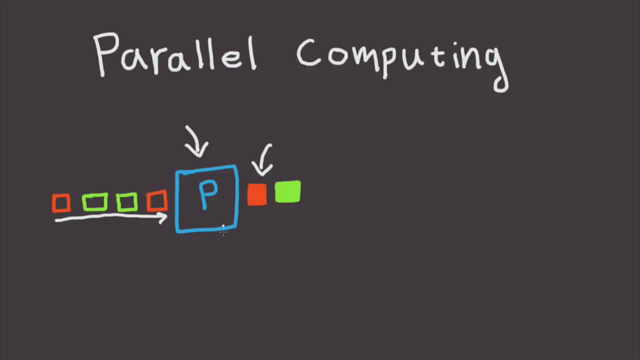 very high and that's one of the reasons why we can't really increase the speed of processors at the one single processor, because it will melt down. So because of this reason we had to take a different approach. so if you want to increase the speed, but 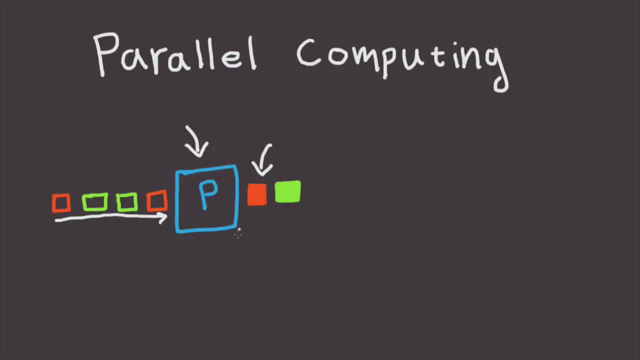 we can't really increase the speed in one single processor because of heat. then what can we do? So one thing we can do is to increase the number of processors. this way, we have two processors running simultaneously and we divide the tasks between these two processors. this is: 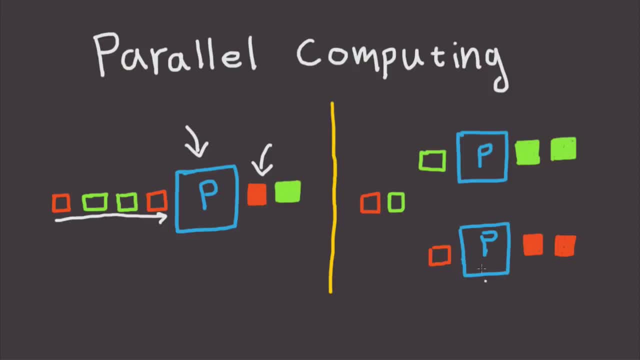 called parallel computing, two processor running at the same time doing the calculations, and we divide the workload between these two processor. of course, this introduces a new set of potential problems, and one of them is more bugs, because you should know when first which instructions you need to divide and 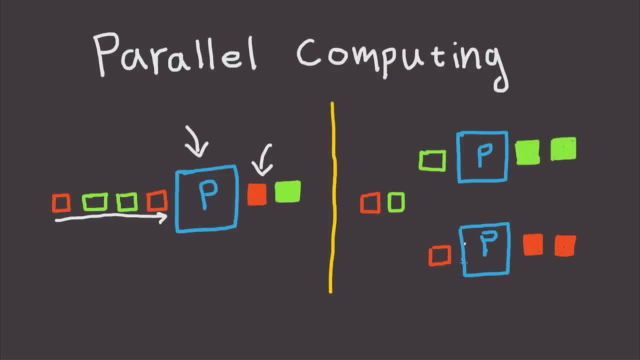 what instructions need to be dedicated to each of these processors? because let's say that you assign a kind of a process to this processor here and that task gets done fast, but this task is dependent on a process which is currently being run by the other process here, so you can have a kind of a